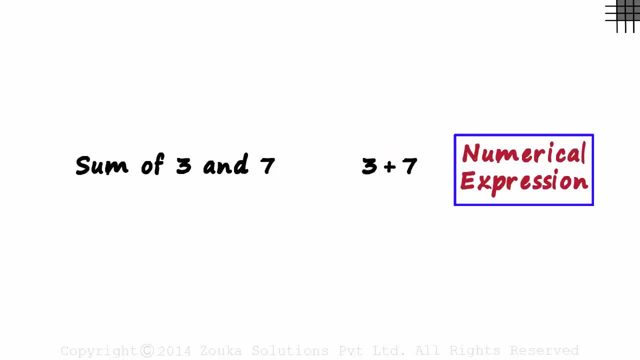 Only numbers, numerical expression. Now how do we write the sum of a number and 7 in a mathematical way? As we don't know what this number is, we can use a variable in its place. We can write it as x plus 7, where this x can take any numerical value. 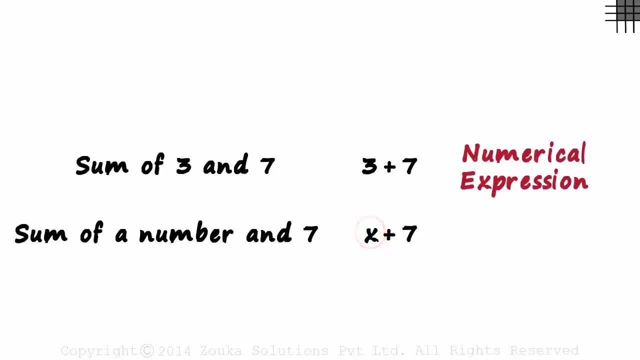 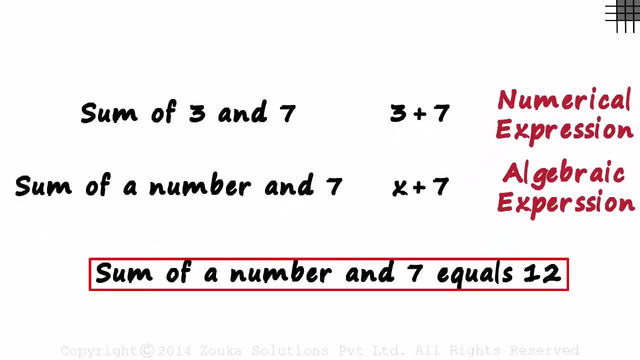 As this expression also has a variable in it, it's called an algebraic expression, Variables. then algebraic, just numbers, then numerical. Here's another statement. we need to write in a mathematical way The sum of a number and 7. 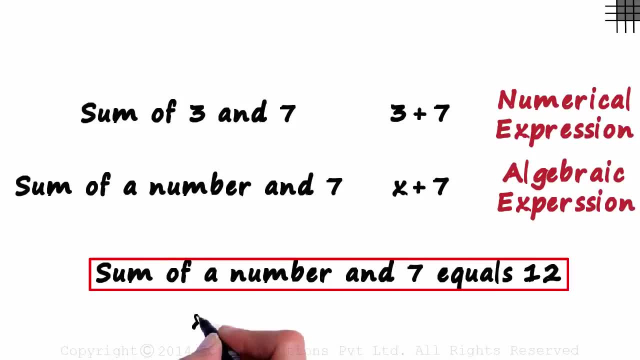 equals 12.. This can be written as: x plus 7 is equal to 12.. A number plus 7 equals 12.. This is called an equation. It has an expression on each side of the equal to sign. Apart from expressions and equations, 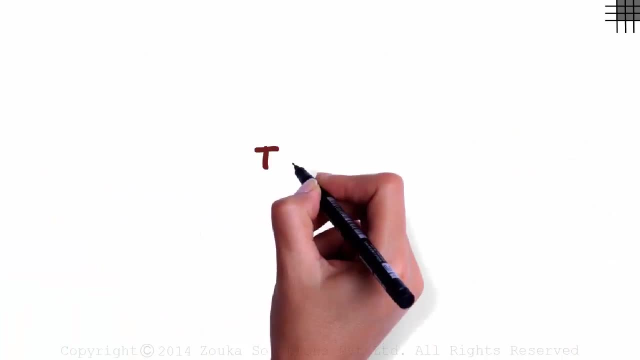 the most important concept in this topic is that of terms. Look at the number 4.. It is just one term. What about 4 plus x? How many terms do we have in this expression? Two terms: 4 and x. What about the expression 4 over x? 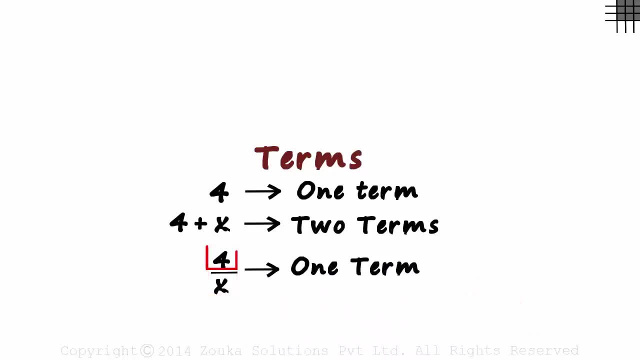 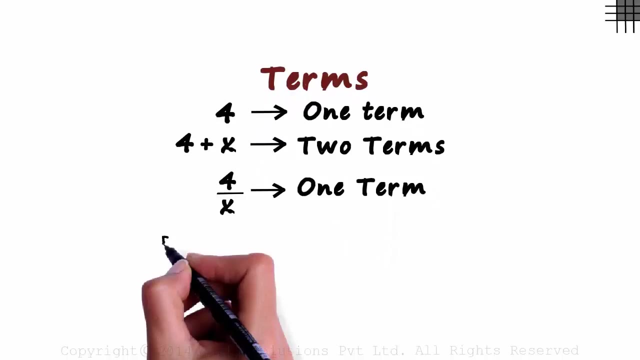 This is just one term. One term when divided by another, gives us only one term, Not two, Only plus and minus. separate the terms Multiplication and division do not. So here's the fourth example: 4 plus x, minus y, As we have plus and minus. 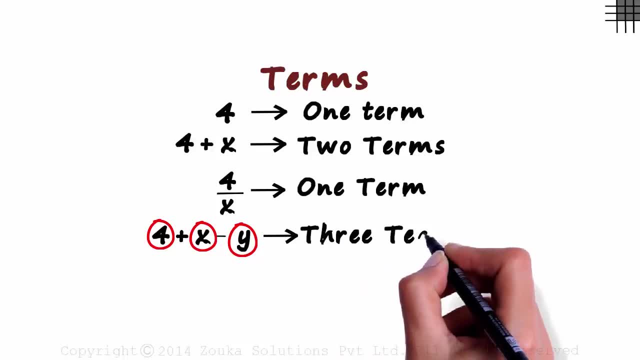 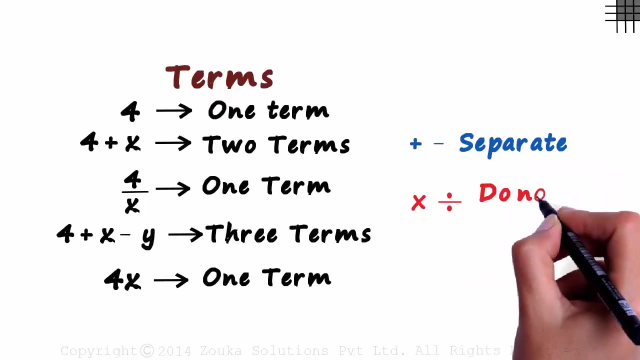 we can say that this expression has three terms. And what about 4x? As 4 and x are multiplied? this is just one term. So remember: plus and minus. separate the terms Multiplication and division. do not What are like and unlike terms. 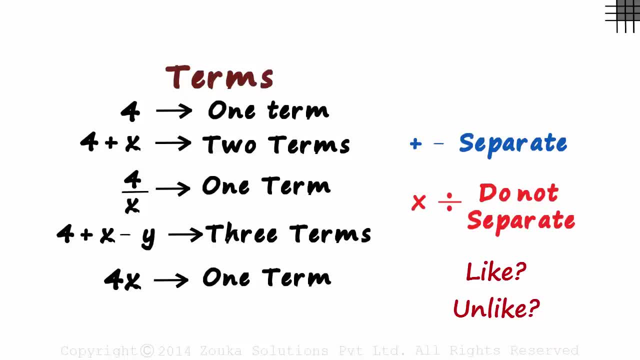 We will see that in the next session, Thank you.